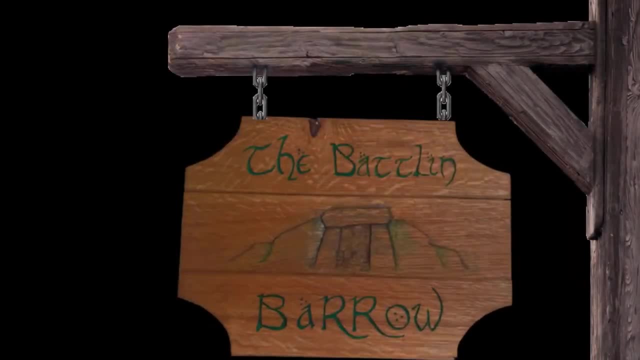 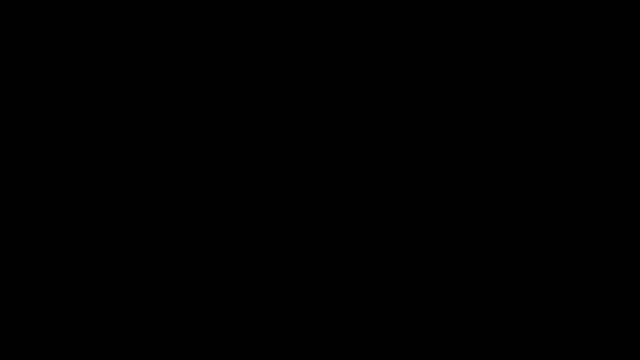 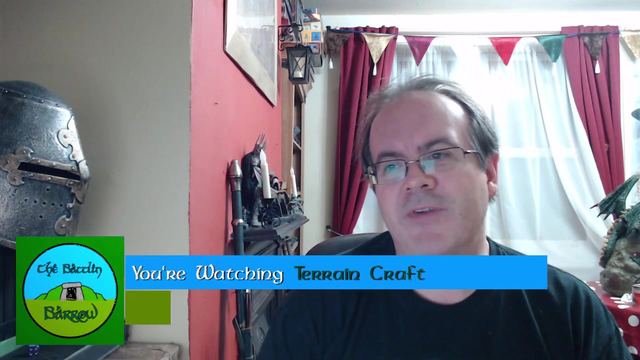 Let's do something a little different with this craft. Hello and welcome to the Battling Barrow. My name's Kev and in this crafting video we're going to do something a little different. We're not going to make any terrain, but what we are. 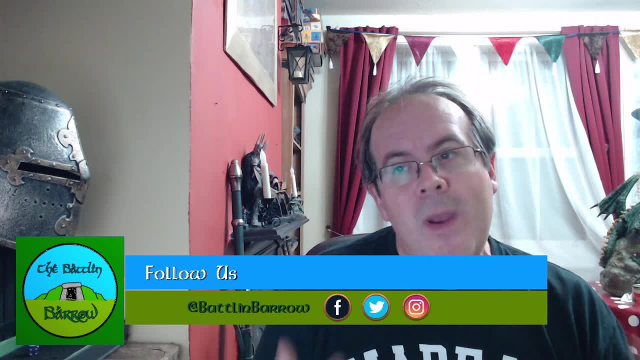 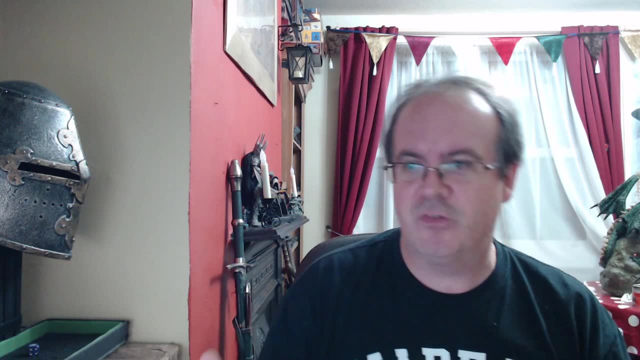 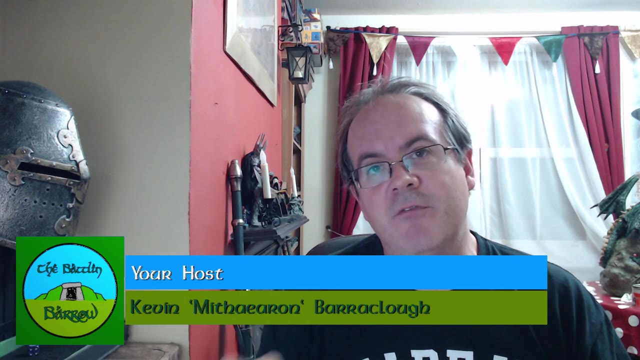 going to be making are some game eggs. When you are playing board games and tabletop games, you soon get swamped with cards and tokens and board sections and whatnot. Pretty soon, your play area will become a mess. What you need is something to manage this. You could, of course, buy something off. 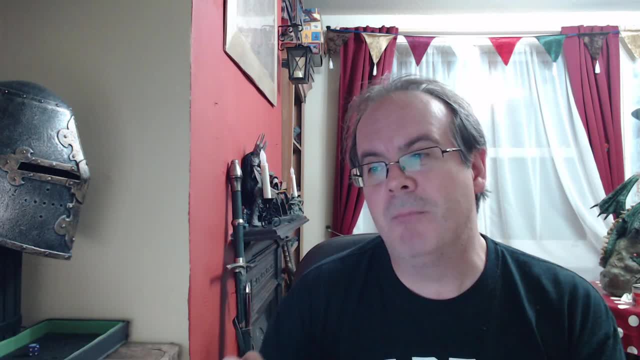 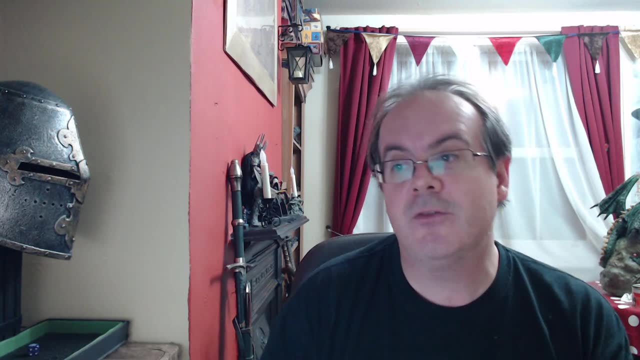 of Etsy or, like nowadays, most likely 3D print something. But if you are like me and enjoy crafting and the crafting experience, you're gonna want to make something yourself, and that's where this video comes in. We are going to make a game that's going to be a little bit more fun. We are 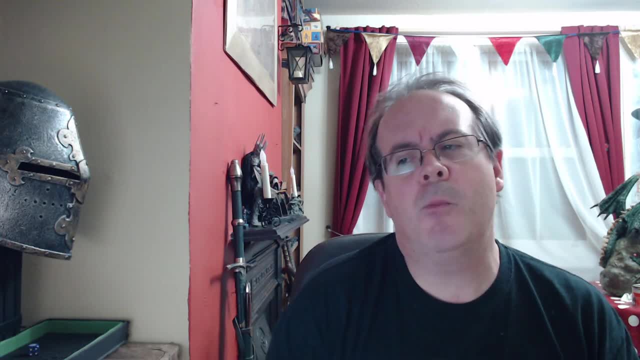 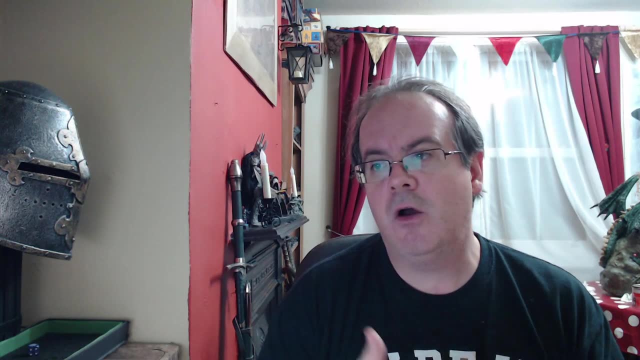 going to make a game that's going to be a little bit more fun. We are going to make a game that's going to craft four gaming aids to help organize and streamline your tabletop play area. We're going to make some card holders of two different size groups: a token holder, a player tray. 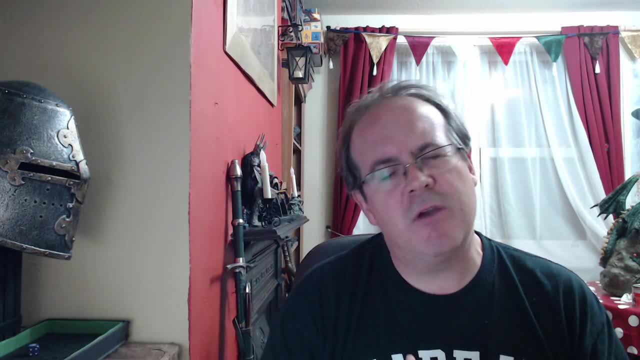 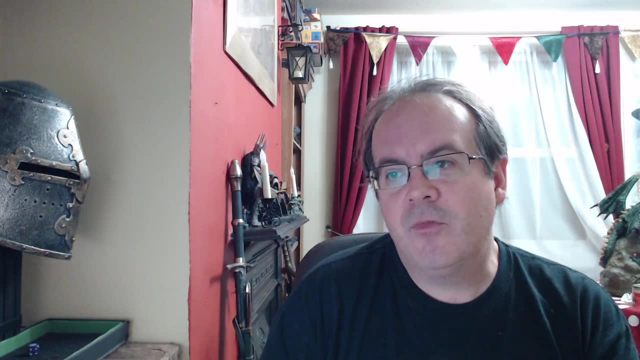 and another that will help you to keep track of things like enemy health. So let's start with the simplest: the card holders. Tabletop games often involve stacks of card decks. dungeon crawlers have dungeon decks, treasure cards and events. Different game systems use. 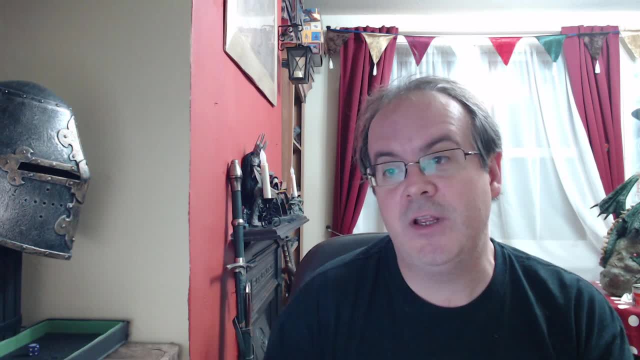 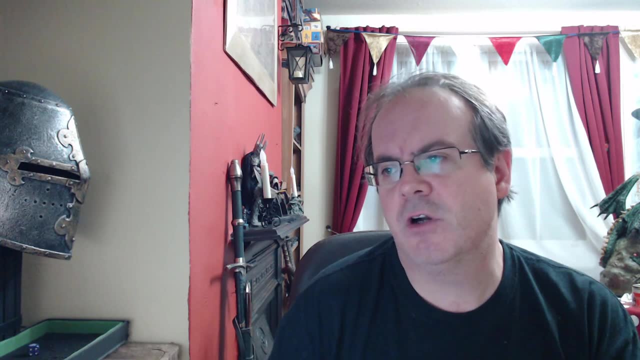 different card sizes, but I've put these together in roughly two groups. There are large cards such as those from Warhammer Crest, Wrath of a Shardalon and Hero Crest. So whilst the cards from each game are not exactly the same size, they are what I will group as large Some games. 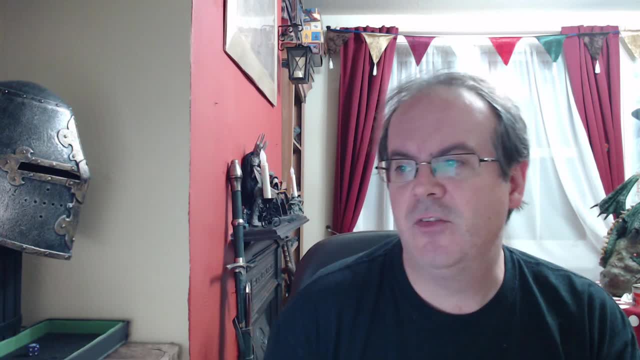 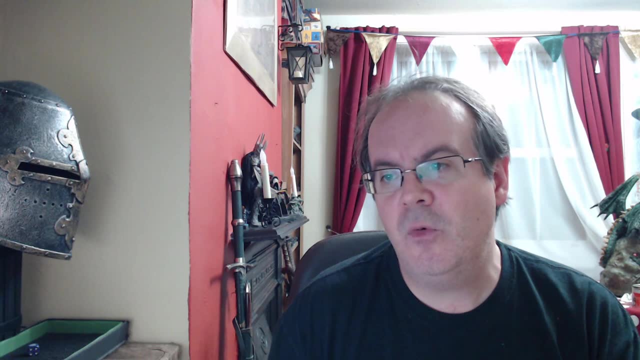 use small cards, such as those from Descent Journeys in Middle-Earth and Talisman. Again, not all of these are the same size, but I will group them as small. So, when it comes to the card holders, I am going to make ones for both groups In this. 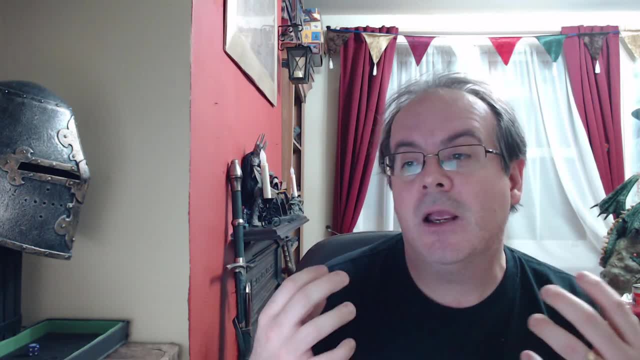 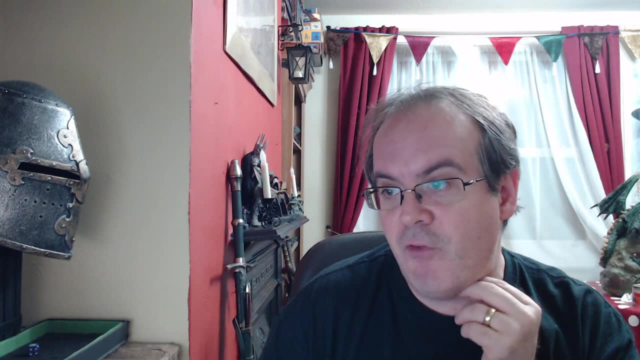 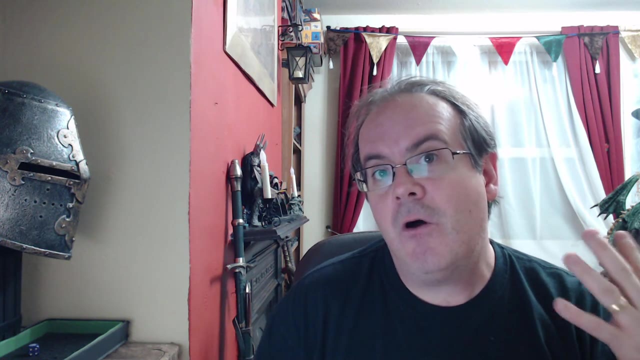 video. I will show the large ones and give a brief overview of the smaller ones. The first thing to do is look at all the games you have with large cards in them and find the largest out of those cards, As if the cards are smaller than the cards that you. 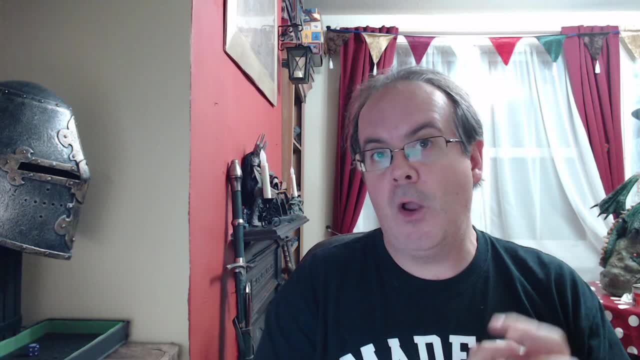 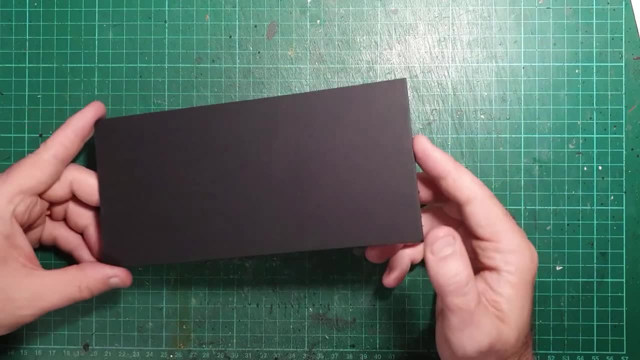 have. If the card holder can hold those cards, it will be able to hold the smallest out of the games you have. I will be making holders in sections with each holding three stacks of cards. So I measure the width of the largest card and multiply it by three, As it will. 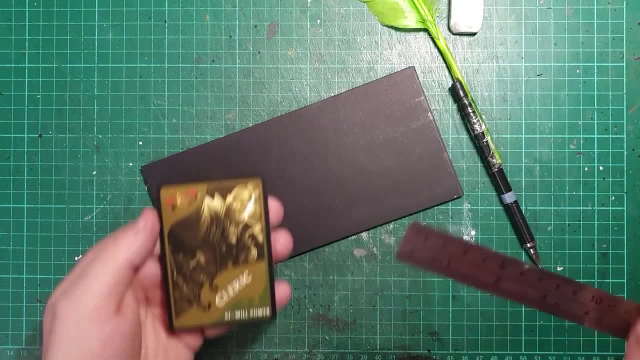 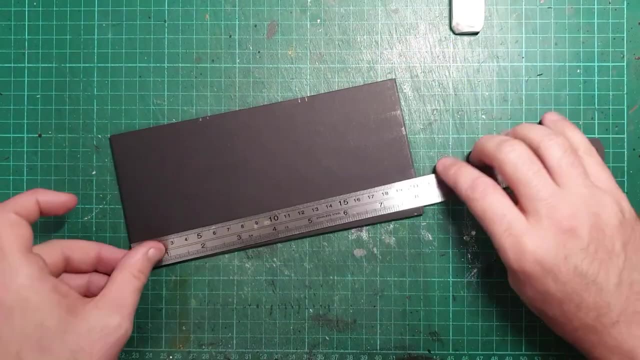 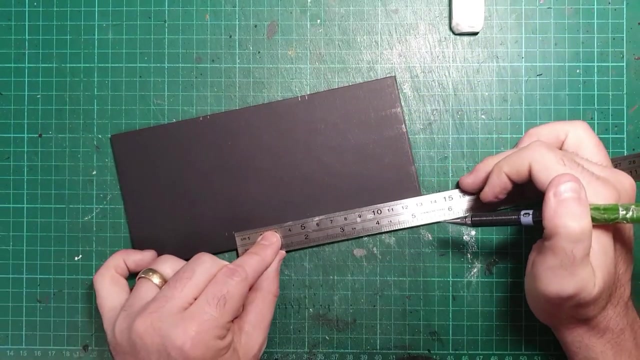 hold three stacks. it will have two dividers, so I will need to add two times the width of the foam core, which in this case is 5mm thick, so 10mm in total. I will also add 6mm for measuring and cutting errors and to allow for a bit of wiggle room. 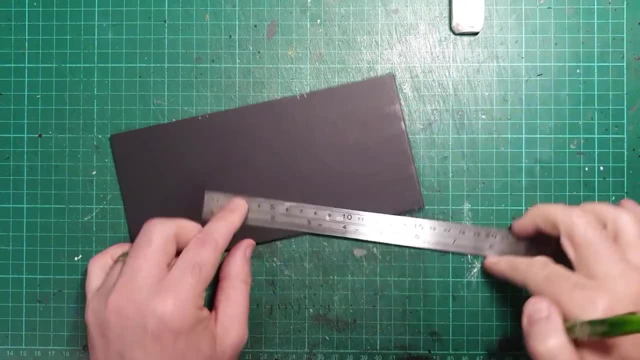 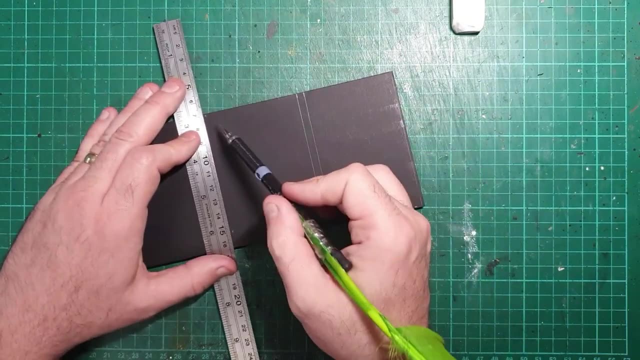 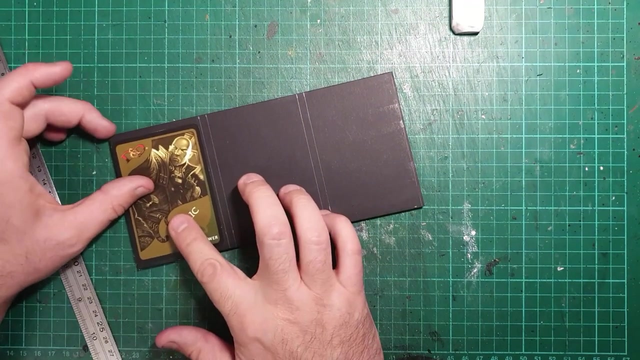 The width of the holder base will be the length of the largest card, again with a few mil wiggle room added. So in my case this will be 220mm by 95mm. This gets cut out Inside. I measure the width of one card plus 2mm, and then 5mm, and then 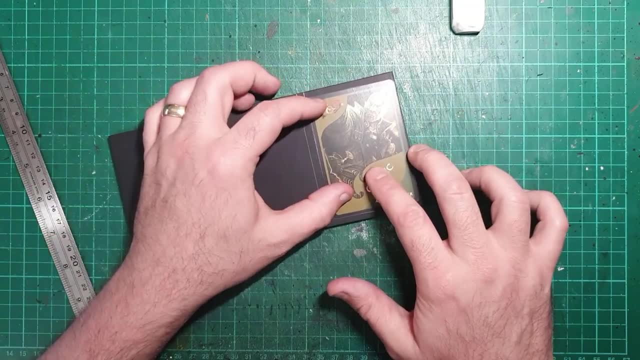 the width of another card plus 2mm and another 5mm. This divides it into two sections. I measure the width of each card and multiply it by into three sections with two dividers. Next I cut out two bits of foam core. 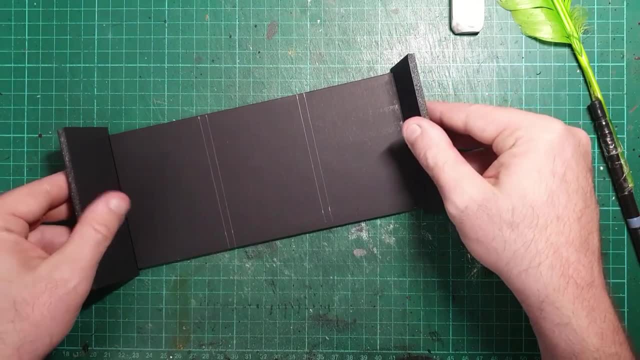 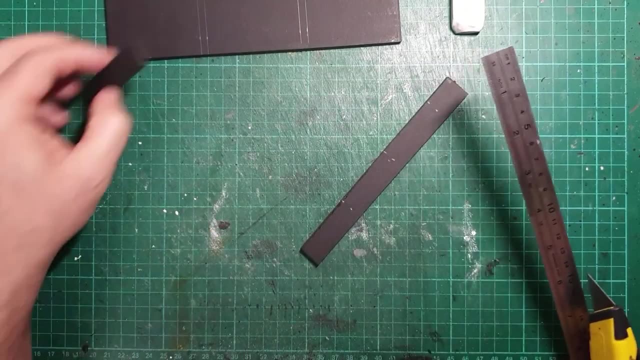 that are 105 mil by 45 mil. These will act as the two end pieces. Eight sections are cut out that are 17 mil by 45 mil. Set four of these smaller pieces aside for now. These are then glued into place. 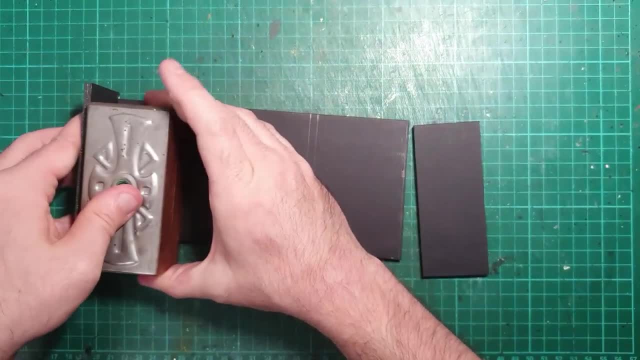 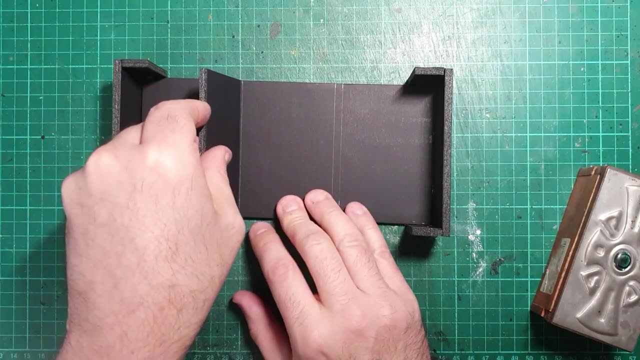 I use a box to help get things straight and at right angles. Two more pieces of foam are cut out that are 95 mil by 40 mil. These will help form the dividers and are all glued into place with the four set-aside pieces from earlier. 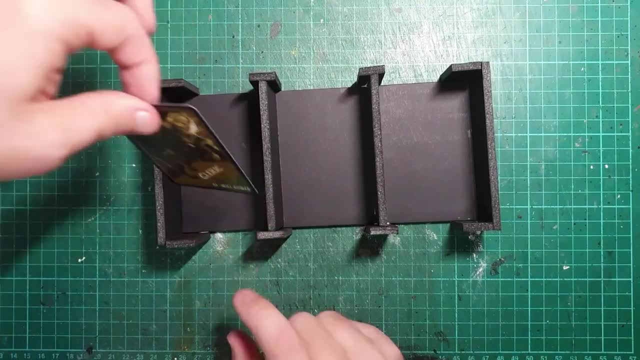 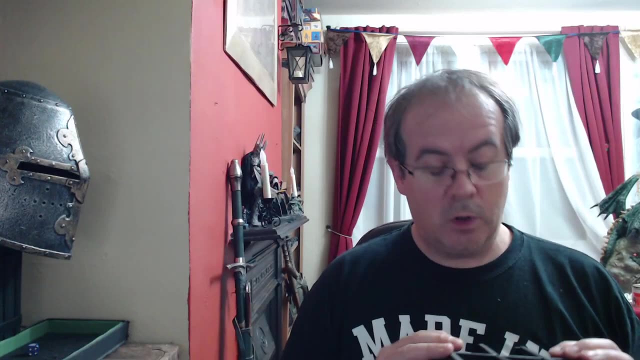 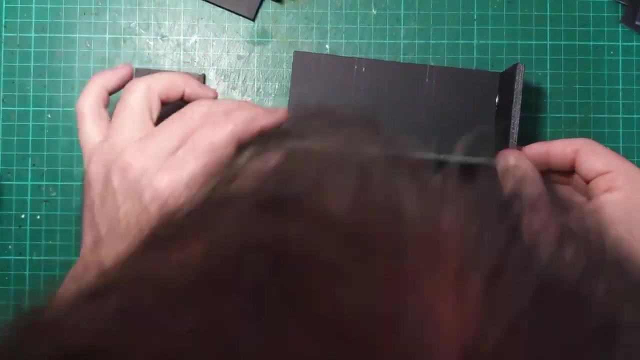 I use a card to make sure it all fits at each gluing stage And when it's done you'll end up with something like this: The smaller card holder is done in much the same way, except it's 13 and a half by 15 centimeters is the dimensions. 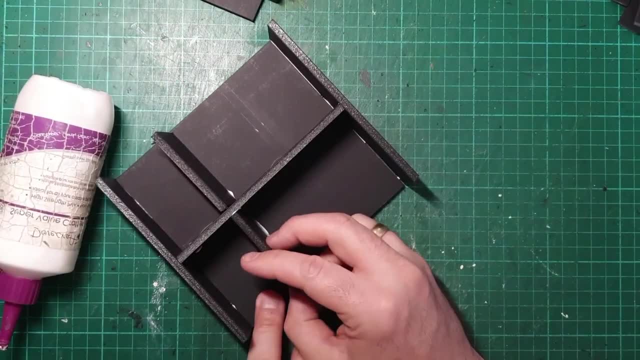 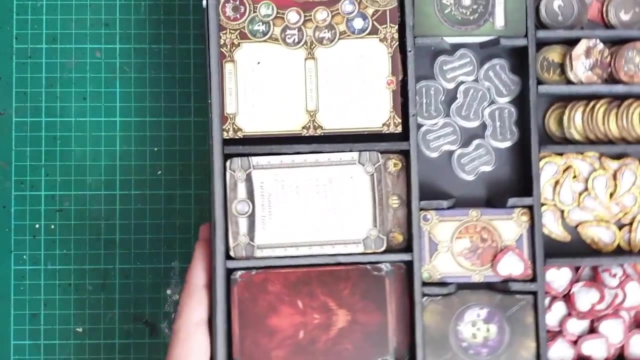 and it holds six cards. And the smaller card holder is made in a central compartment, So it just has a central bit in the middle there, but it's made in much the same way. Tabletop games utilise a lot of tokens and chits. 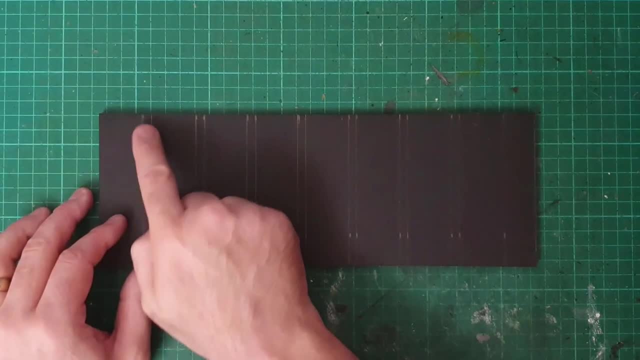 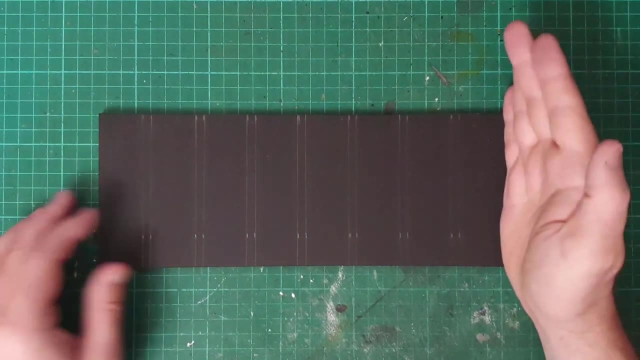 For these I find the best solution is to make trays. I am going to make three: one a long one and two that are roughly half the length. This should cover me for all tokens in most games I have. I'm going to cut in a piece of foam. 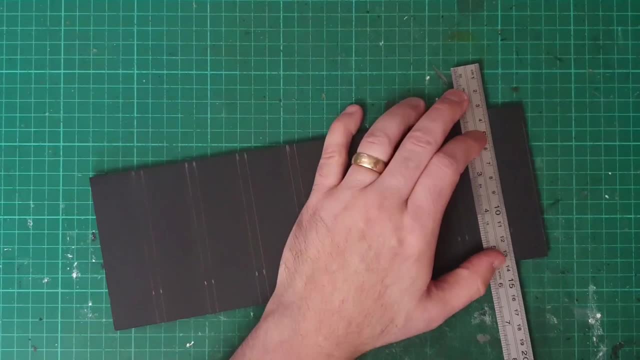 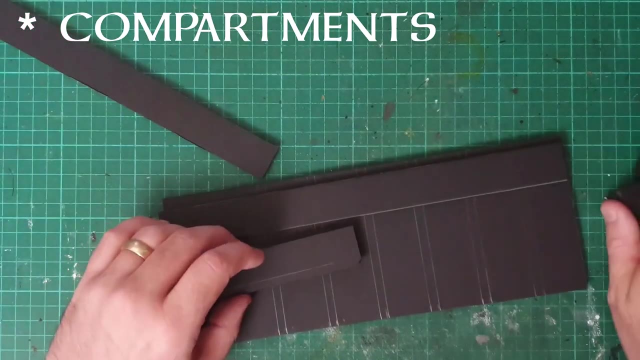 that is, 28 and a half centimeters by 11 and a half centimeters, And this will allow for eight components. It's made in a similar way to the card holders, but it's only two and a half centimeters high to allow easy access to the tokens. 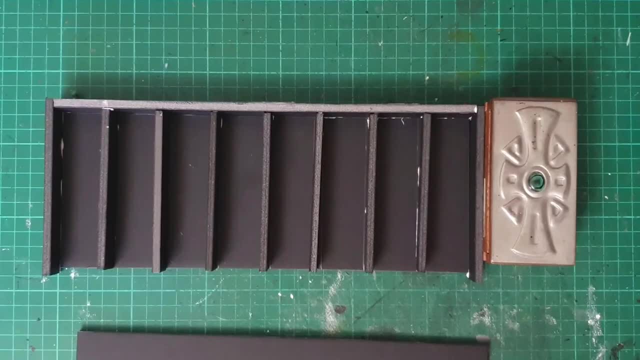 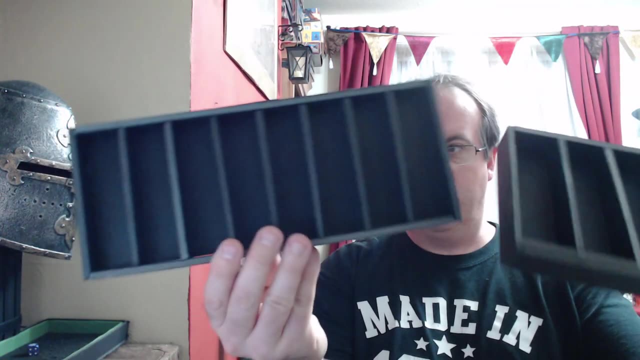 The two smaller ones are 14 and a half centimeters by 11 and a half centimeters and have four compartments, And you'll end up with them looking like this: You have a long one here and you have two sort of smaller ones. I just 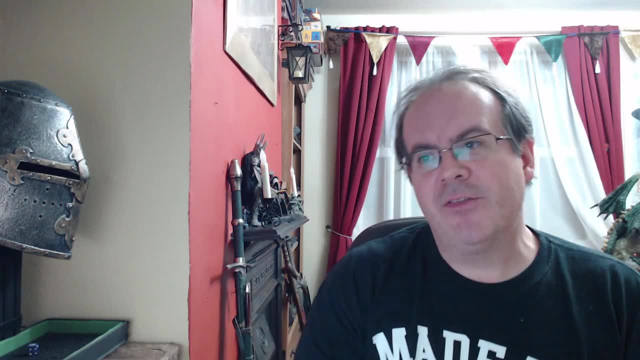 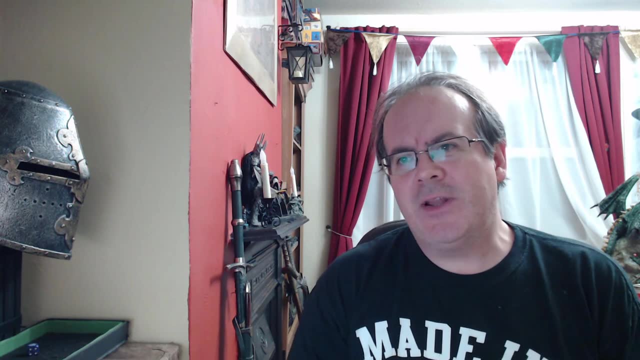 Onto the player mats. Now, player mats are a little bit different, as they will have to be tailored for each individual game for the most part. But even then you can try and design it so it could be used for as many games as possible. 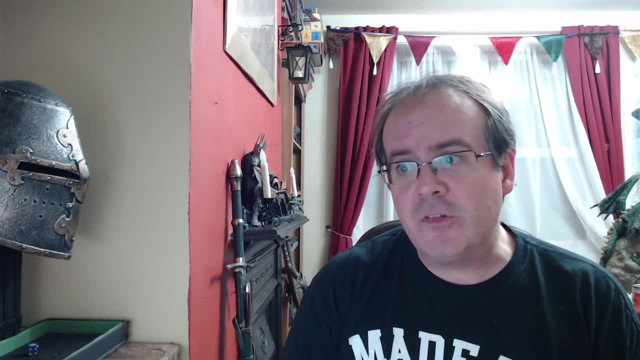 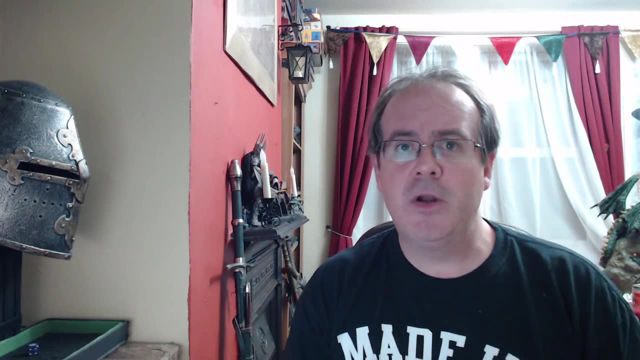 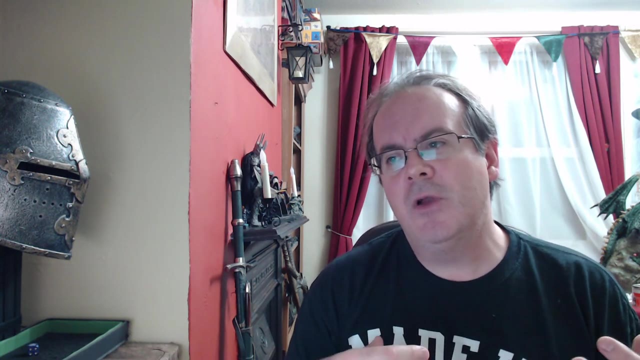 So the one that I will be showcasing here is for Descent Second Edition, But out of push I worked out I could use this for another game as Journey's in Middle Earth. When designing and thinking about the player area, you need to think about how you play the game. 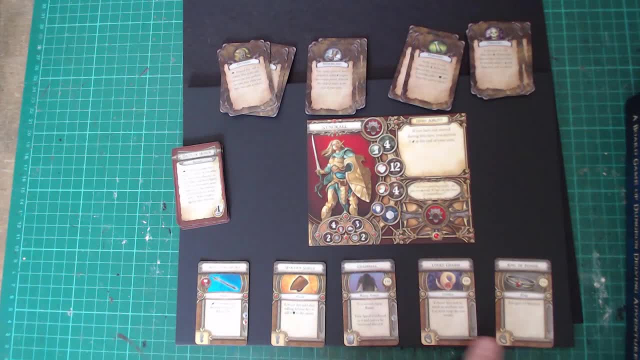 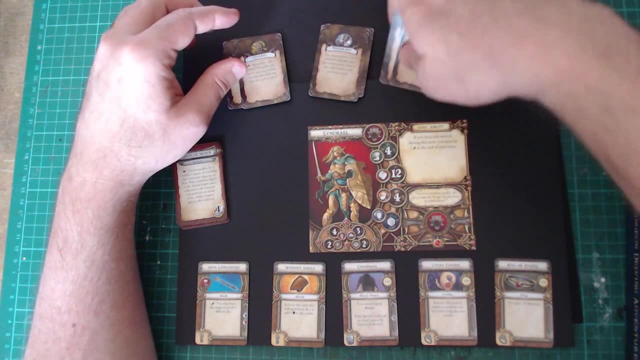 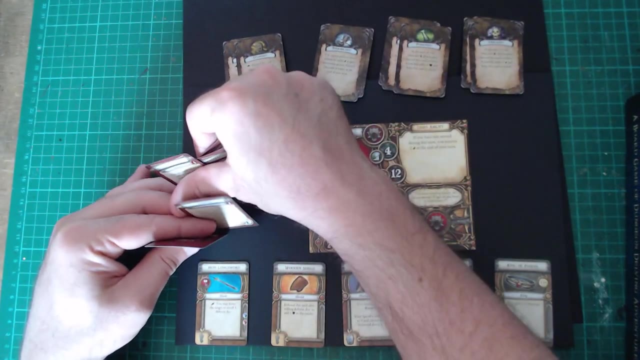 and how you lay out your area. For this one, I wanted to have a player card in the middle. Along the bottom. I want to have an area for equipped items in use. Descent uses both health and fatigue tokens, So I wanted a place for those on the map. 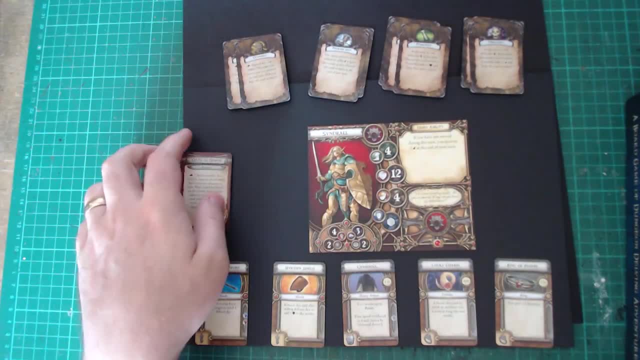 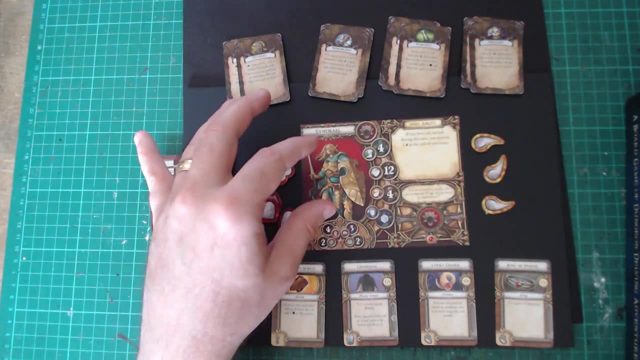 It also uses player tokens, even though I'm using search tokens here when I'm laying it out, So I wanted to have them standing up for easy, so they're easy to see and remove as they get used. Descent also uses skill cards to improve your characters. 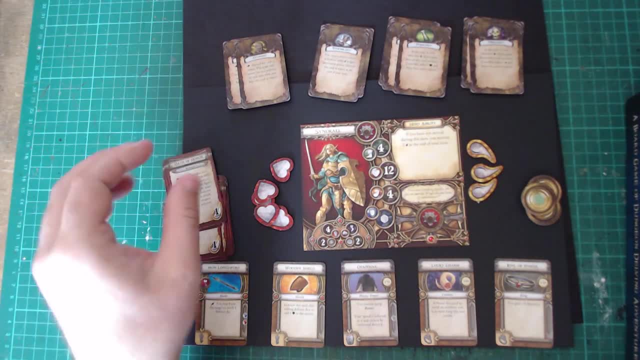 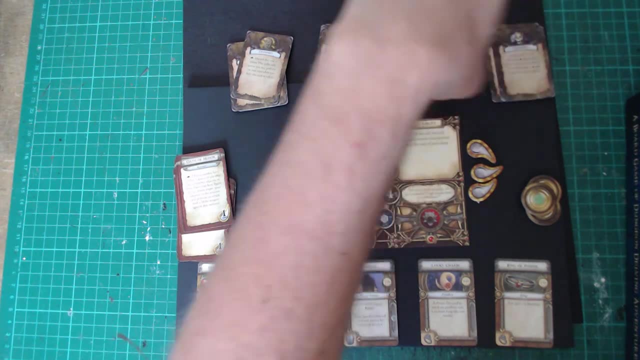 On average, there are about 10 of these per class, So I wanted to have an area for these. The final thing is condition cards your player can have. With that in mind, here's the final design I came up with, So I wanted to have an area for these. 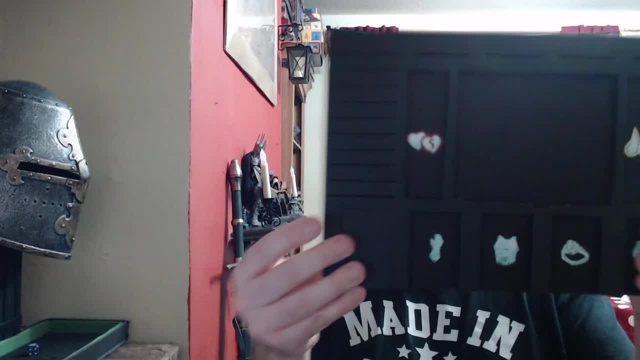 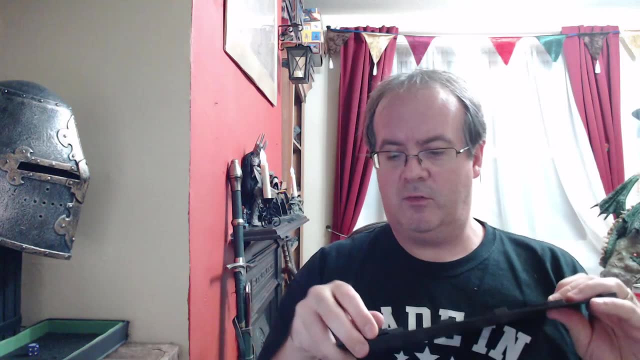 The final thing is condition cards your player can have I came up with, so here it. here is the final design which we'll go over making in a minute. one thing to note is when we get to cut out these, I kept one of these so I can remove it, so you can have two hands, but if you've got a two-handed I 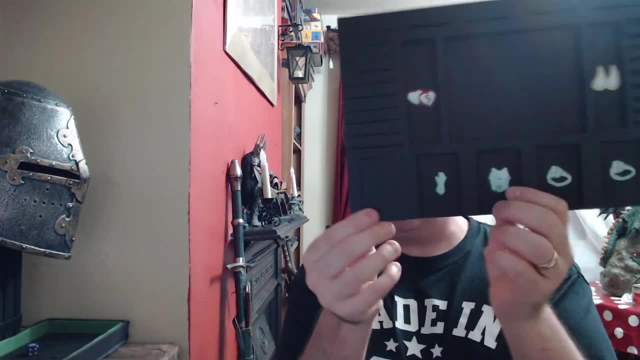 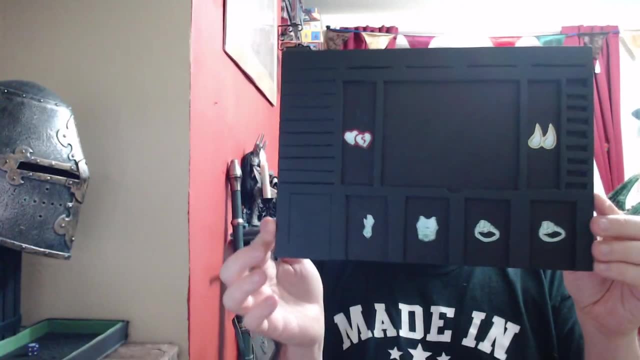 am equipped just as little reminder. you can't equip anymore. you can cover one up and I also just printed out some bits in. but here it is. let's go over making this. this is simply made from foam core and chippal. the foam core is 30 centimeters. 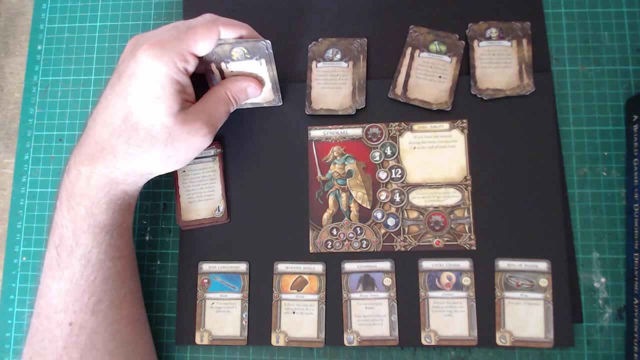 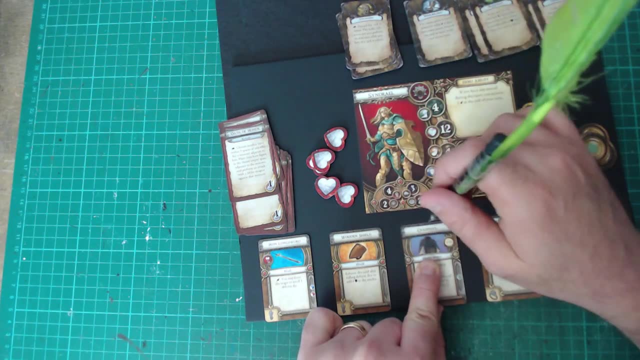 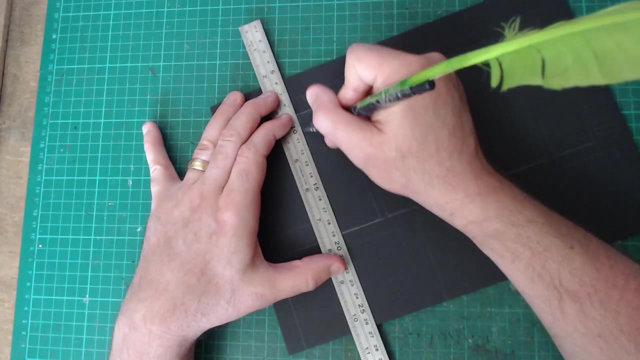 by 21 centimeters and then with the game components I wanted to have on it, I played around the layout. so when I was happy with them, I put them in their place, use the pencils, draw around them and then use a ruler to tidy up the lines. use name shop knife. I cut out the pieces with character sheet. I added a. 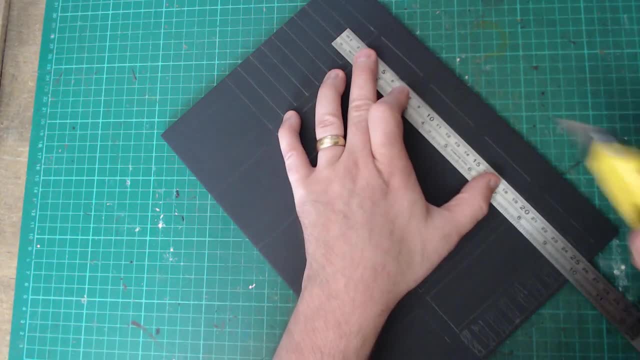 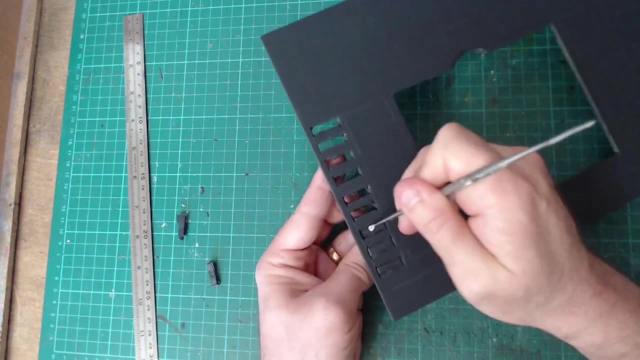 small semicircle to remove the to make removing the card easier. you Bingo. Thanks for watching. I hope you enjoyed this video. The tokens required a little bit more work to cut out and I used a sculpting tool to help push them out. 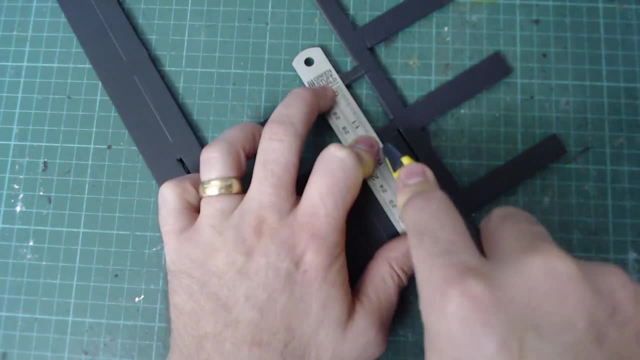 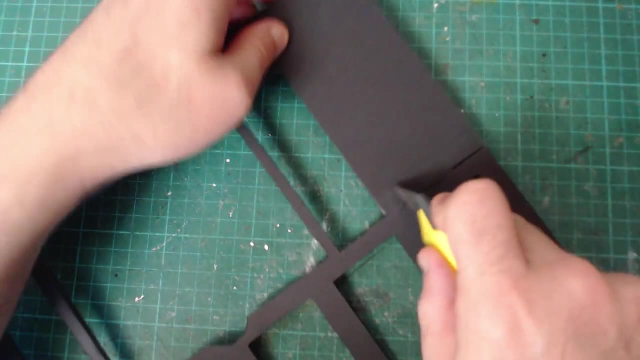 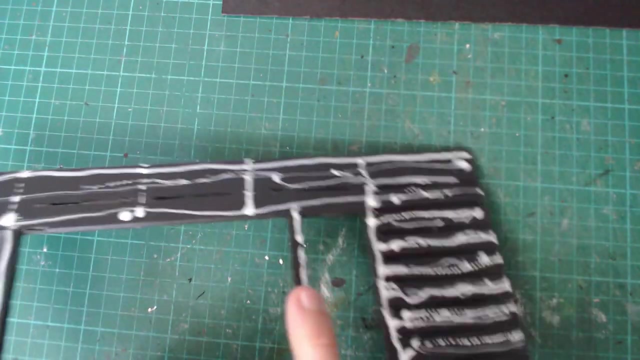 The card slots were done by cutting two lines really close to each other and then just nipping them at the end on both sides. I then used the sculpting tool to push these through. The condition slots were done in much the same way. Once it was cut out, PVA glue was applied to the back and placed on a piece of chipboard that had been cut to the correct size. 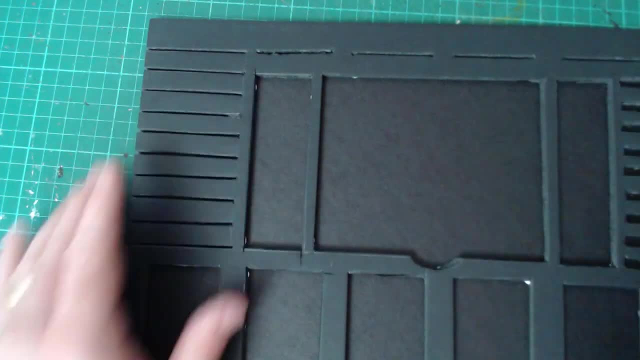 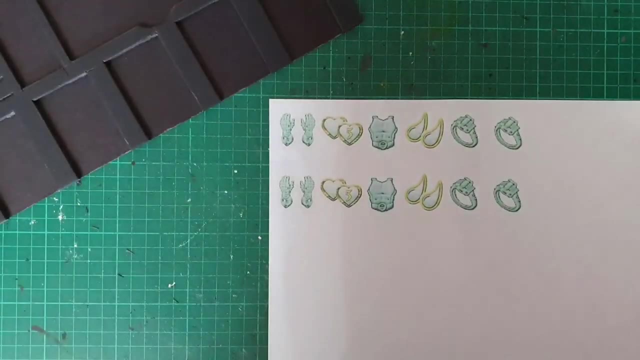 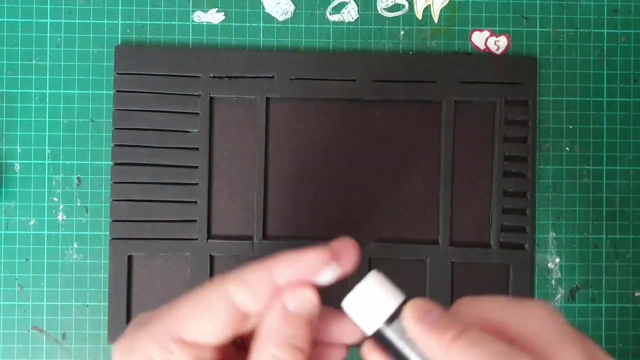 Some heavy books were placed on top. whilst it dried, I printed out some artwork for the health, fatigue and equipment slots on paper and cut these out Using a glue stick. these were glued into place. My printer was running out of ink so I will probably reprint these at a later date. 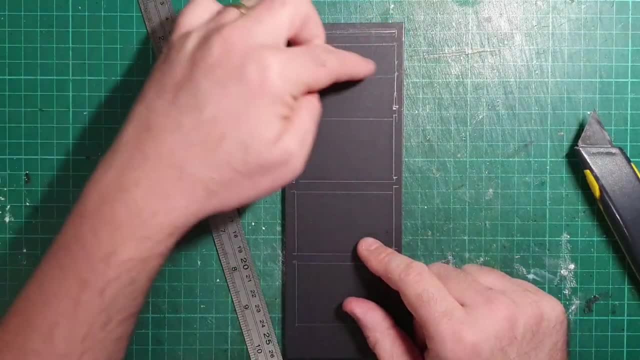 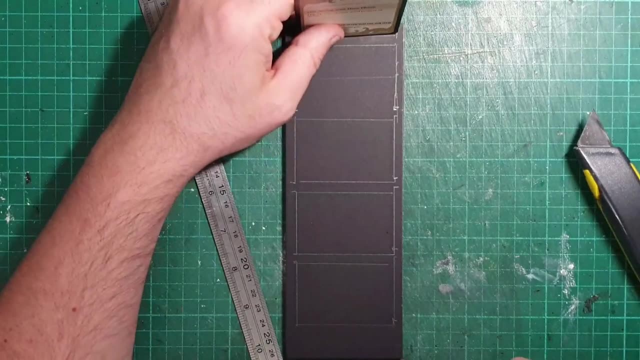 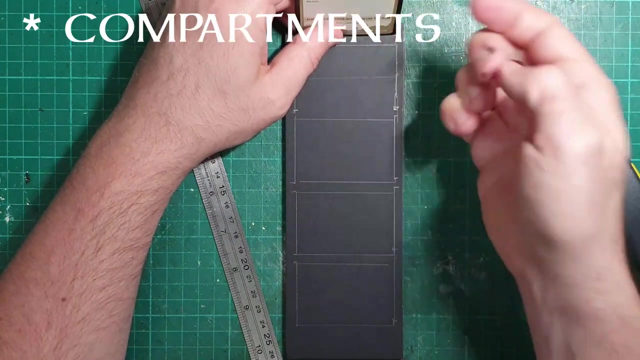 Now onto the Enemy trackers which I have here. I made four of these and they were designed with Descent 2nd Edition in mind again, Although I guess you could use it in other games. It's got a slot at the top here so you can put your card in the monster card and then different components to put their health into. 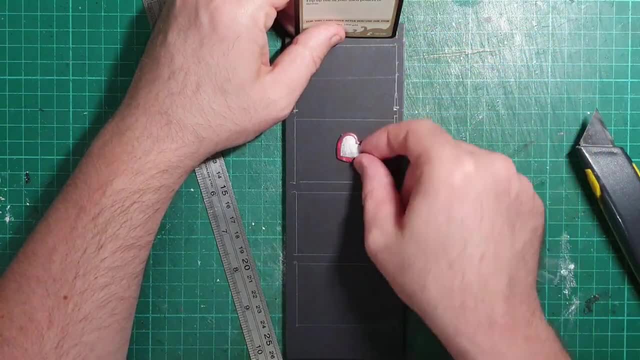 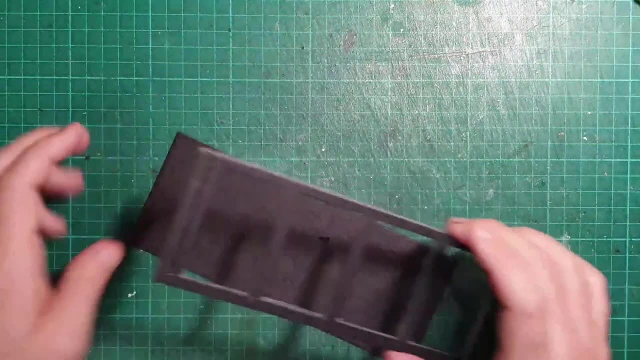 But even if you had a game like Wrath of a Shadowland that has an environment card that is sometimes always in play, you could slot it in there and you've got your environment card in there. You could slot it in there and you've got your environment card in there. 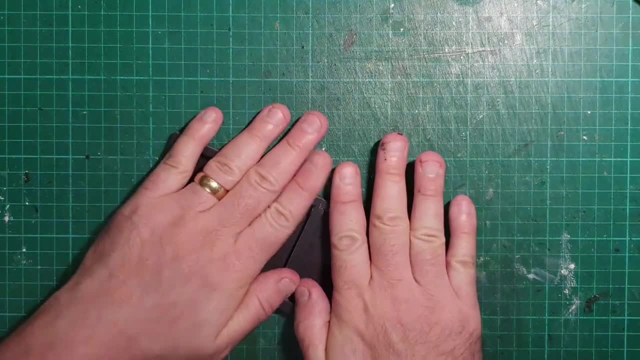 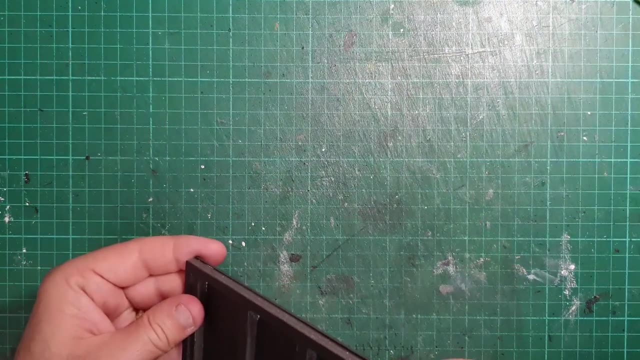 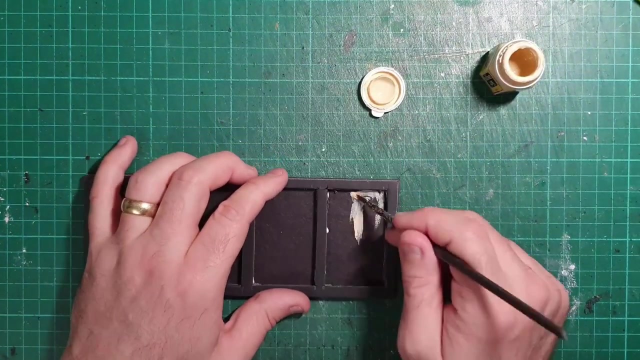 The environment card has a reminder. Each of these is 19.5cm by 7.5cm And, as mentioned, you've got a slot at the top and the four compartments. Once it was cut out, much like the player tray, it was glued onto some chipboard backing. 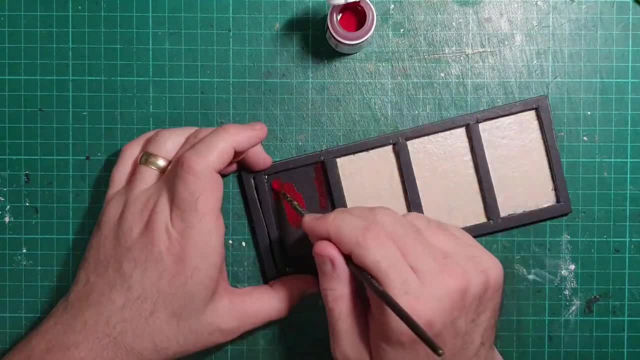 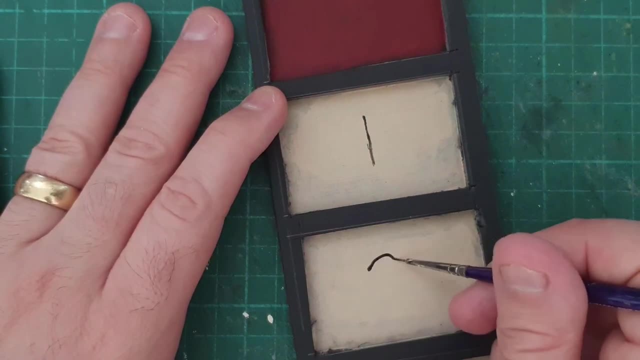 I painted the three minion compartments a cream colour and the top one a red for the master. I then painted numbers one to three onto the minion slots And my minions underneath their base have. each one has a number on it, so it could correspond to the numbers on here. 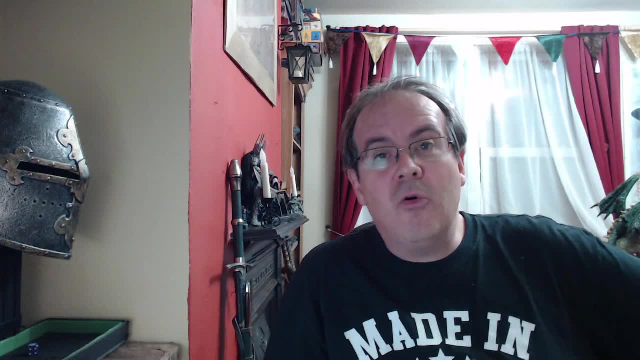 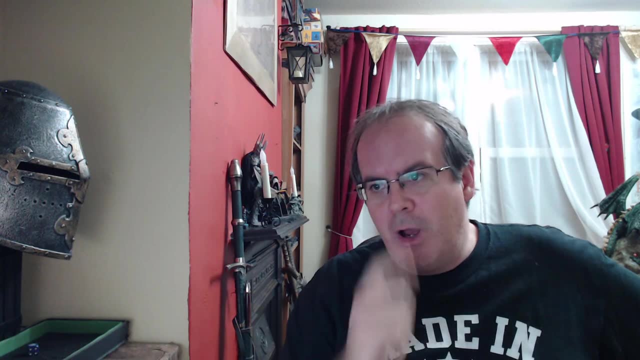 And that's it for game aids. These things are not going to win any best looking game aid awards or anything, But they are practical and really useful. I may have a think about the overall finish and see if there's anything I can do to make them look a bit better. 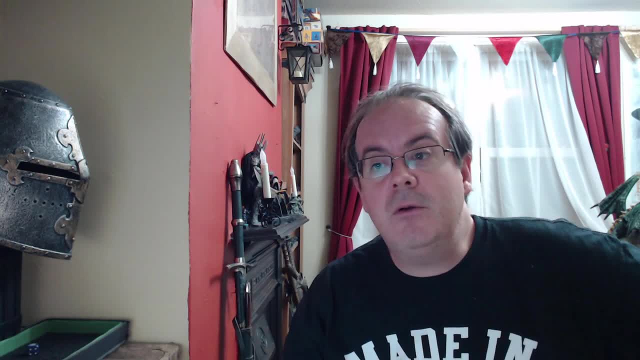 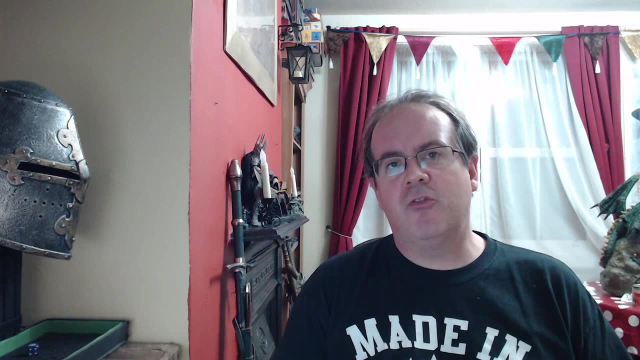 If you have any suggestions, leave it in the comments down below The general game aid stuff, like for the cards and tokens, that's all well and good, But the player trays are probably where it really comes into its own to keep your play area handy. 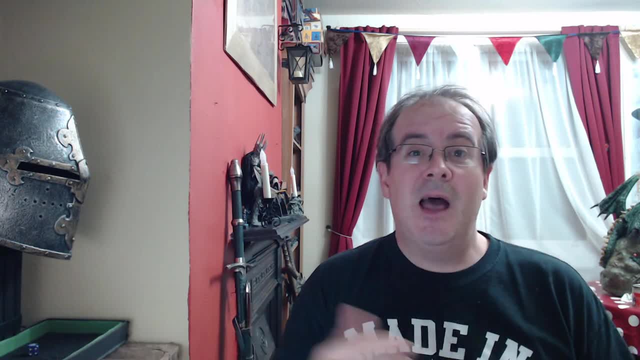 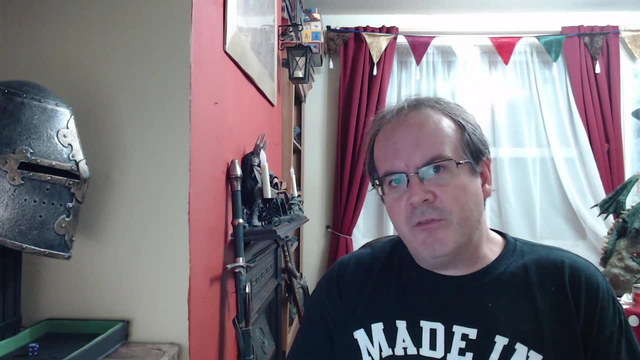 So I may have a think about what other games I play and what other trays I can come up with, And if I do, I may do some follow up videos of just doing a load of player trays. If that's something you'd be interested in again, let me know in the comments. 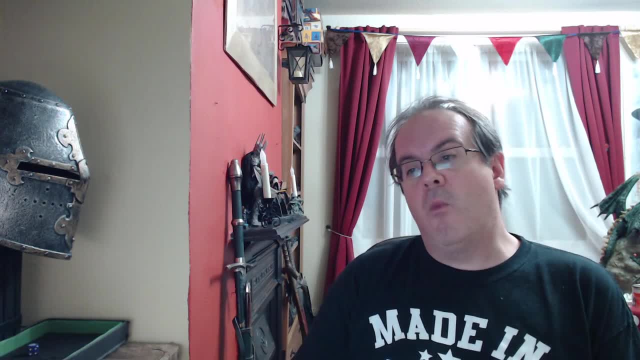 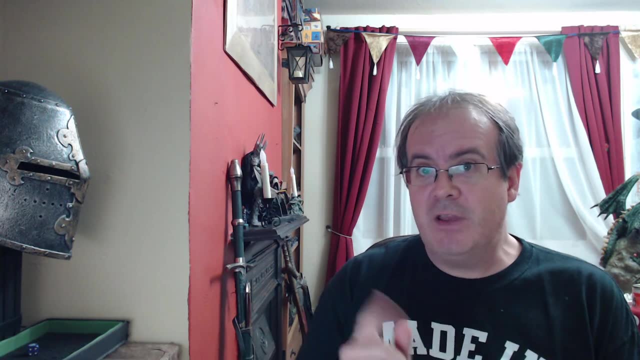 Anyway, that's enough waffle for me. Thank you all for watching and a massive thank you to all my Patrons, who you know, allow me to buy things like Foamcore and things like that. So a big thank you to you guys.